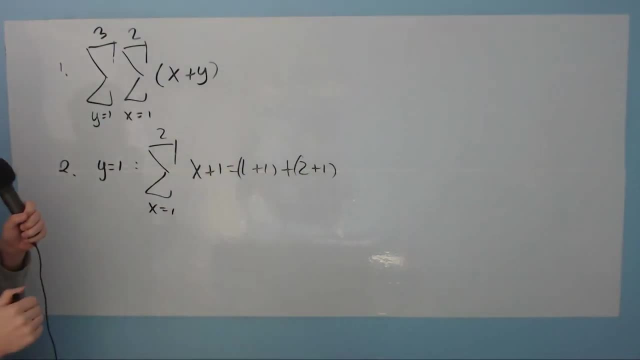 value of one like that. So let's simplify this when I carry this out. let's see, this is going to give me here two plus three, which is five. So that's the first step. We have to repeat this a couple more times. this is only for y equals one. Remember y goes from one. 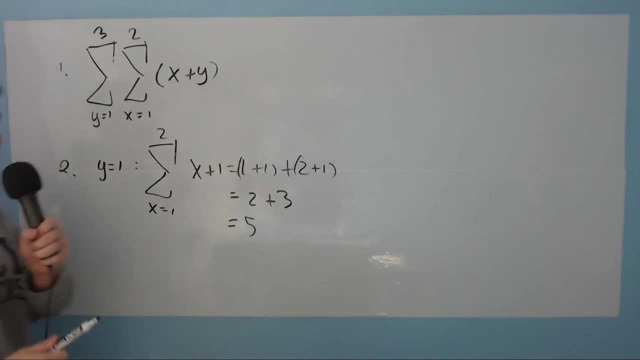 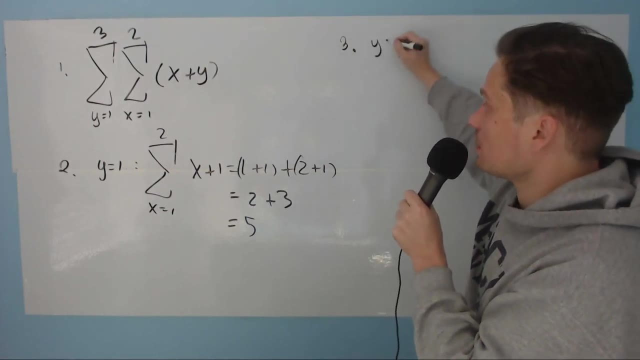 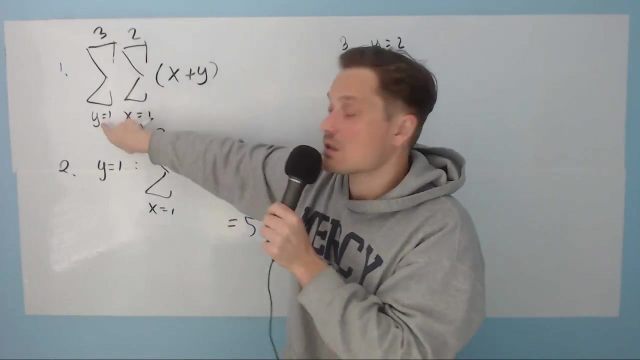 up to three. So then you repeat this logic as follows- Let me move over here to the other side So I can fit my writing Step three. basically, you then said y equal to two, Over here in the outer summation where it says y equals one, two, three. that means you're going to go through a 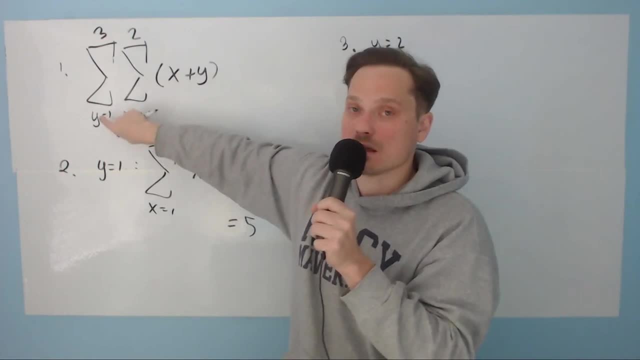 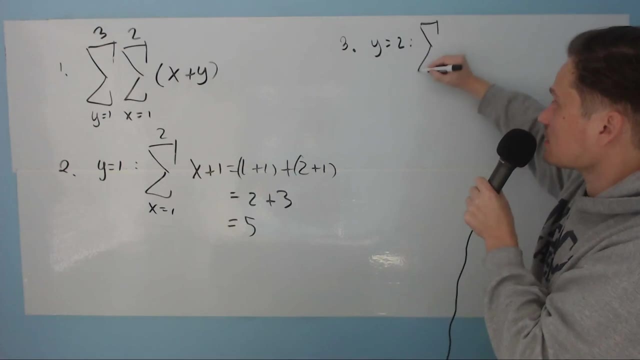 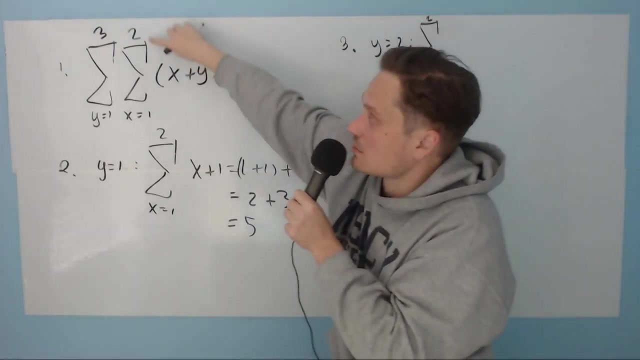 value of two. it goes: y equals one, y equals two, y equals three. So over here at this stage I'm writing y equal to two for that reason And then iterate over the x's. So that means x still goes from one up to two, Because I made it up like this: the inner sum here is two and the 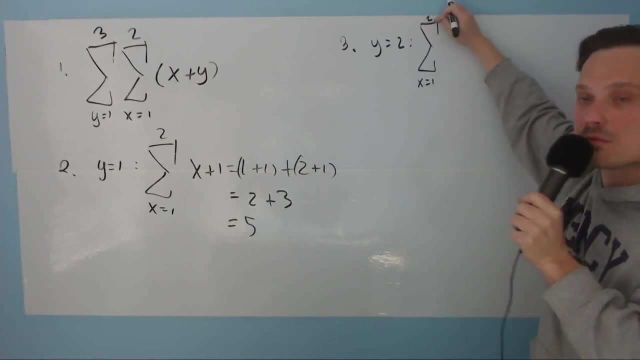 upper value. So up here there's a two present, a little bit small, but I think you can see it still- And then you replace y with this value, So it becomes x plus two. So where I see y in my expression, x plus y, I replace it with two. I'm setting y to the constant two and I iterate over the x's. 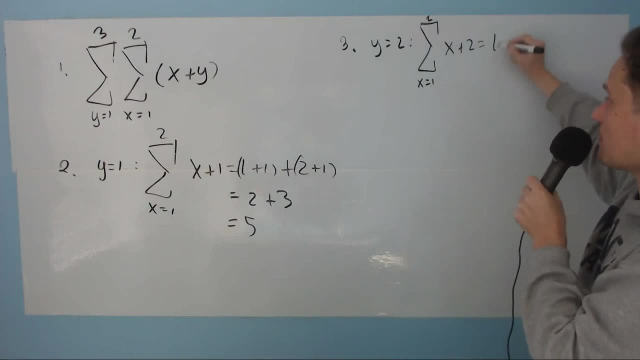 So when I do that, I'm going to have the following here: take a look, I'm going to have one plus two plus, and then after that I will have, of course, two plus two. I simplify this, So this is: 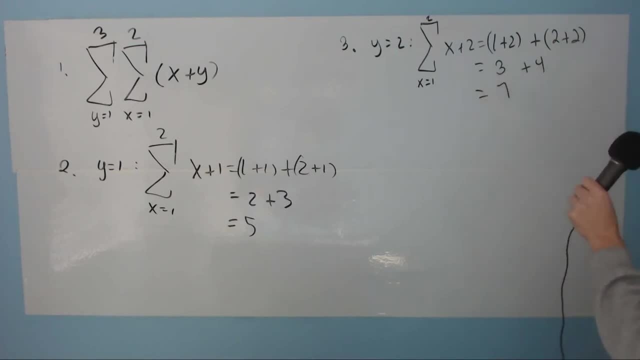 three plus four, which is then seven. Now you really should pause the video and try the next one on your own. I'll do it, obviously. So that's step number four. These are my step numbers. I like to number my steps. I think it makes a difference in terms of how easy the work is to 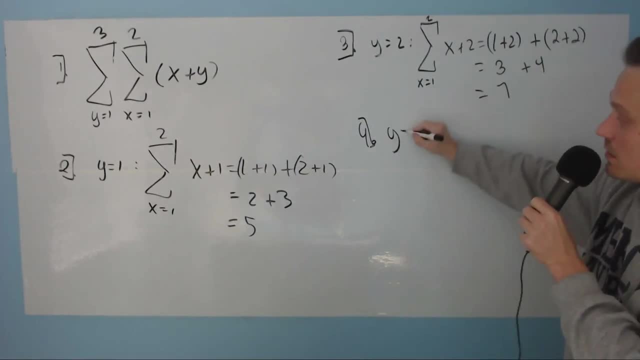 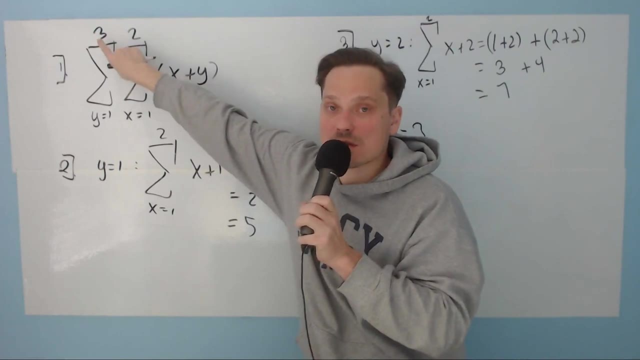 complete. So step number four: I'm going to set y equal to three, and I am doing that y because up here the upper limit for the outer summation symbol, as you can see, is three. That's why I'm. 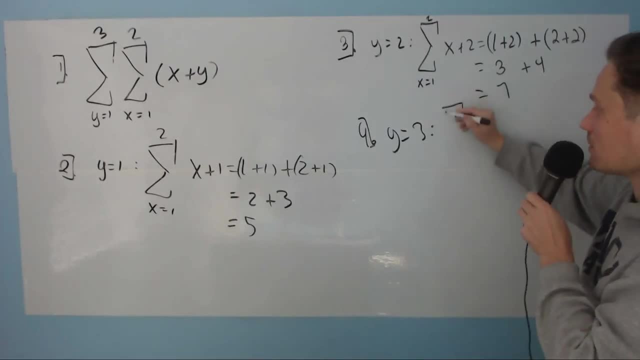 doing that. So I'm setting y equal to three and then I iterate over the x's with that value of y fixed at three. So when I do that, I will have the following expression: now x plus three, And again x goes from one up to two because we designed it that way. I don't mean to mix things up, So here: